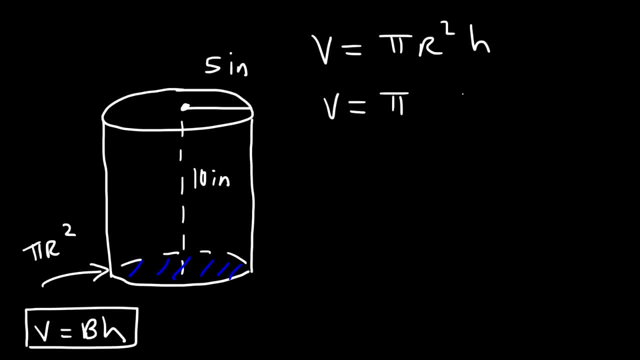 And so it's pi? r squared times h. In this example, the radius is 5, and the height is 10.. 5 squared is 25, and 25 times 10 is 250.. So the volume for this cylinder is 250 pi and it's cubic inches. 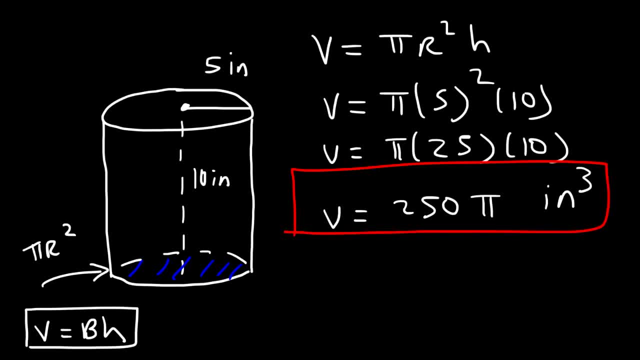 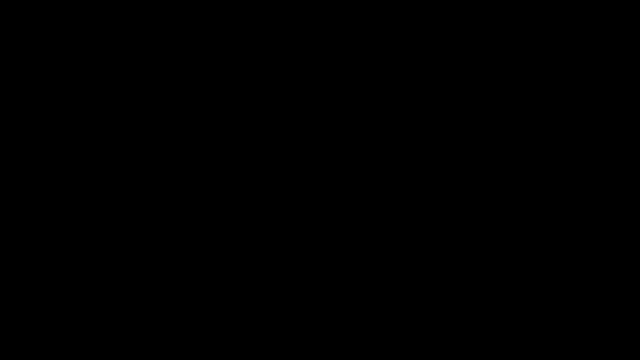 So that is the answer. Now, if you want to get the decimal value of that answer, it's approximately 785.4 cubic inches. All right, So there's actually a number of offensive questions here that will be answered. What is the bard? the Tyrell question. 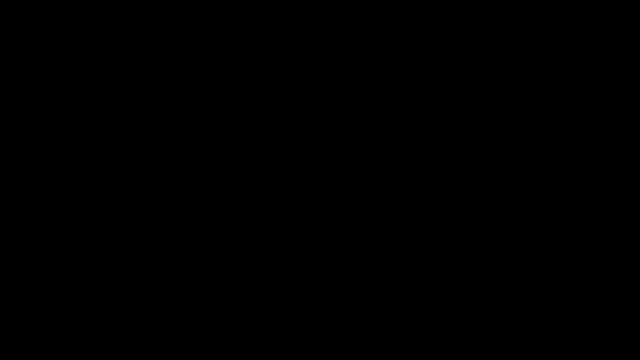 1, 2 squared times 1 squared 7 things. So this is the riddle for the problem of P mu: squared, It's negative. 2 squared times 4. squared It's negative. 2 squared times 2 squared. It is in a bad way. It's the real problem. It is the dumb thing, But the problem is that you are trying to go away, And so what they're trying to find here? they're trying to distort, they're trying to plot things to solve problems. and you're going to Prepond systems, you might have to evenかった them. It's a kind of well, so just to move. did they ask you to write things together?